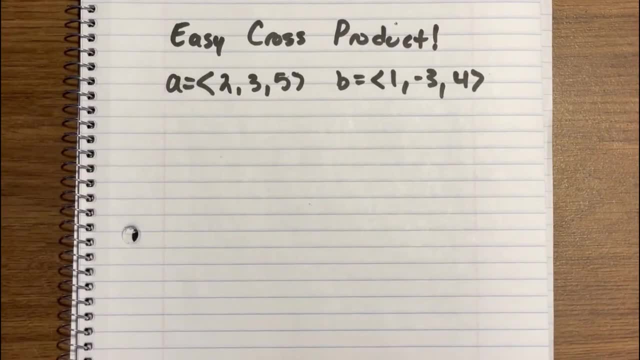 Hey guys, it's Matt. Today I want to show you guys a really easy way to do vector cross products. This is the way that I learned how to do it. It's like a shortcut Instead of drawing the whole determinant of a matrix stuff like that's a pain That takes so much time. This is a nice little. 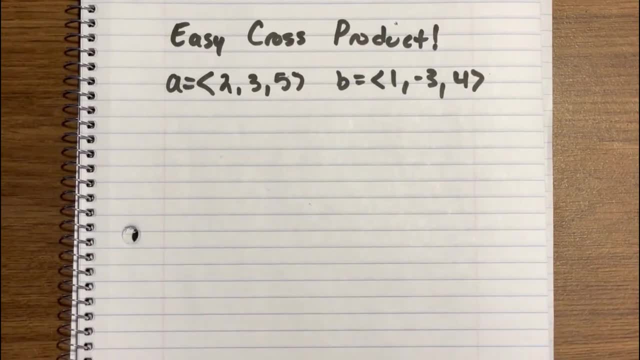 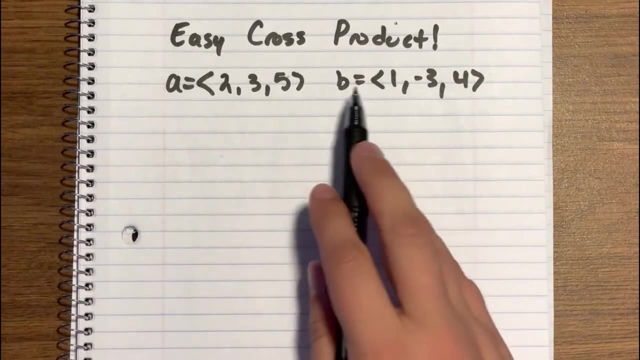 shortcut to make it take a couple less steps and make it really simple. So the first thing you got to do, like we got these two vectors right: A is 2, 3, 5, and then B is 1, negative 3, 4.. So the 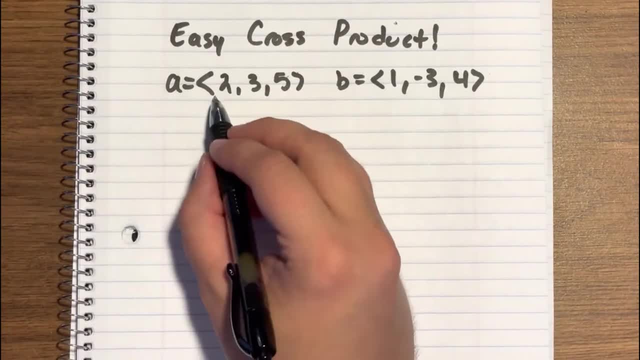 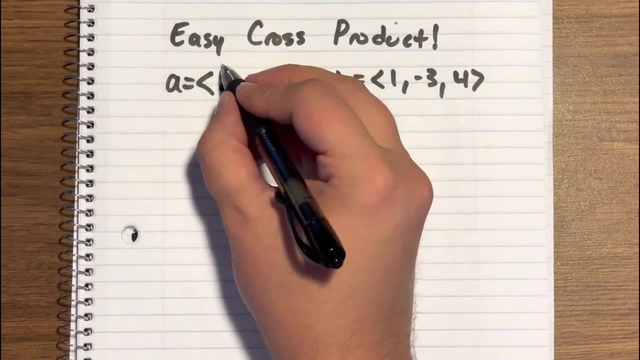 first thing you want to do, like step 0, so this is the A vector and we've got 2,, 3,, 5, right, Remember, the first term is going to be- I, That's what we're going to call this- The second term. 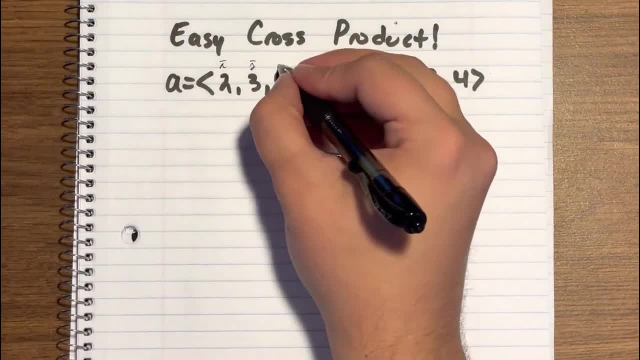 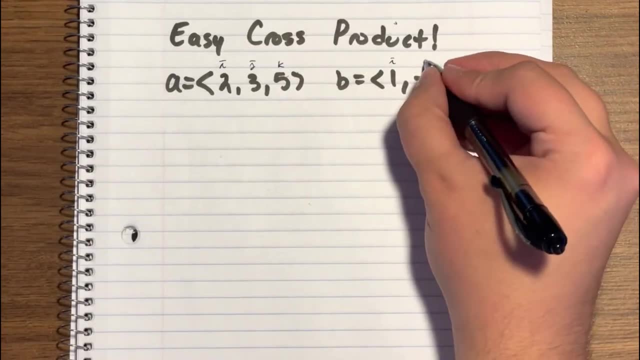 is going to be our J and then the third term is going to be our K And with B, same deal. First term is I, second term is J, third term is K, I, J and K are unit vectors. 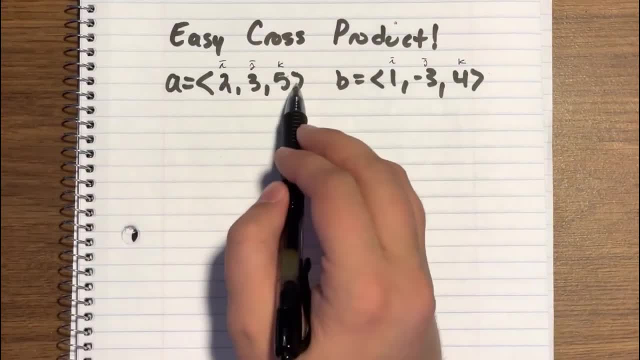 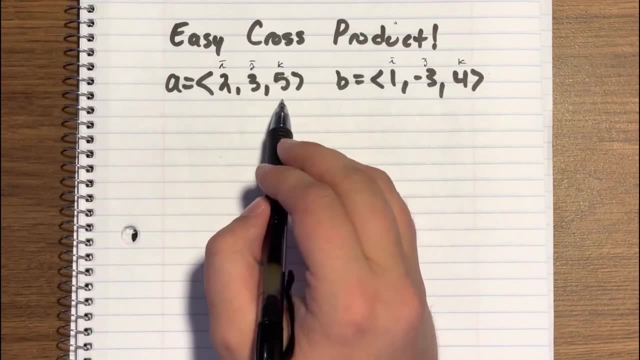 in that direction. So sometimes you might see this as X, Y or Z, but we're going to use it as I, J and K, right, Because this could be 2X, 3Y, 5Z. We're going to look at the I, J and K form. 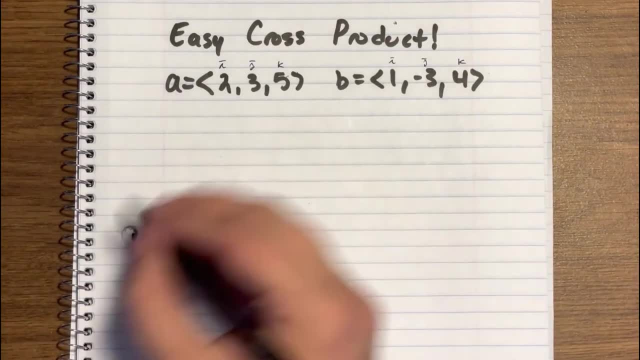 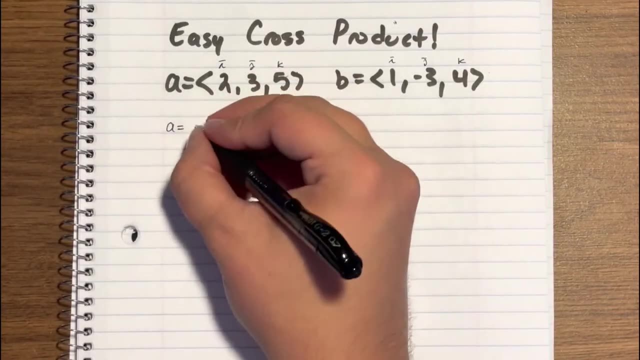 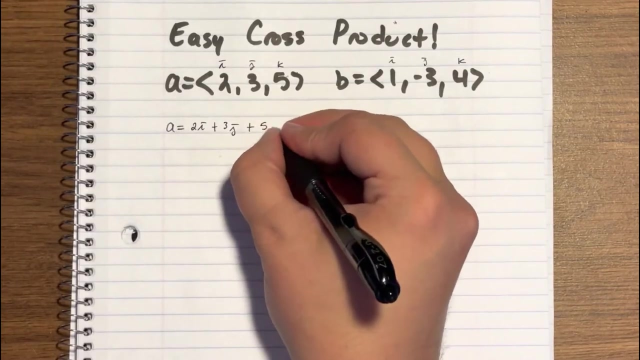 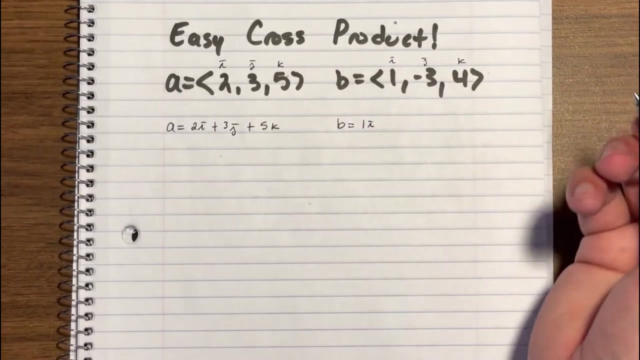 It doesn't really make a difference. This is like the standard, though, So we're going to rewrite this A, This A vector. we're writing it really quick: A is 2I plus 3J Plus 5K, Cool. Now B is going to be 1I. He only has one I. That's kind of sad. 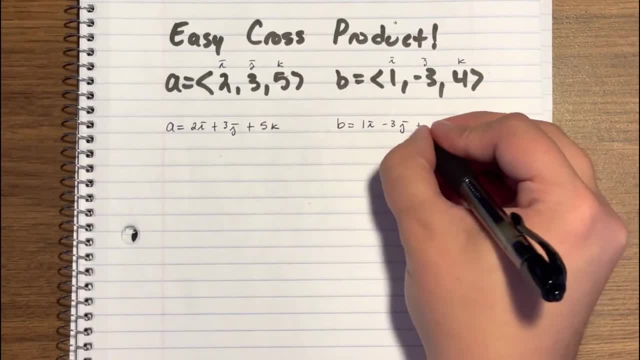 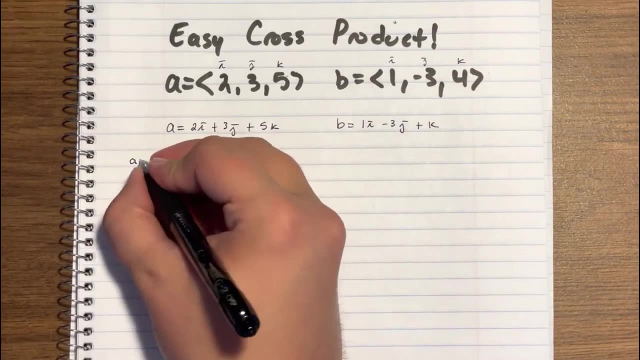 Minus 3J and then four whole Ks. Wow, Cool. So to do this cross product which, remember, looks like A X, B. That's not an X, That's a cross Very different. It's not an X. 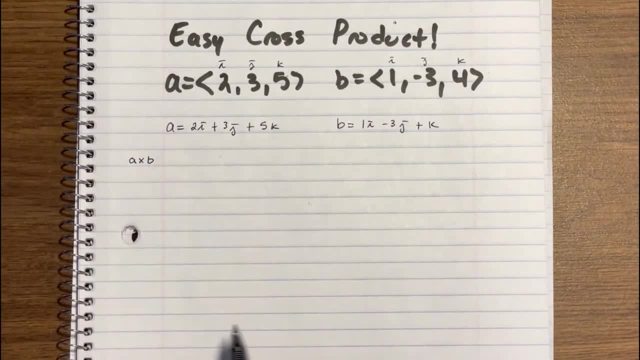 So that's like part of why you don't want to use X and Y and Z and stuff, Because, yeah, it gets confusing. I, J and K, you can't mess up. There's no like A, I, B, right, I mean there's. 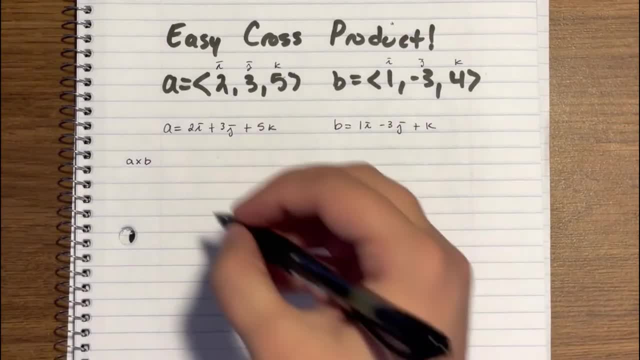 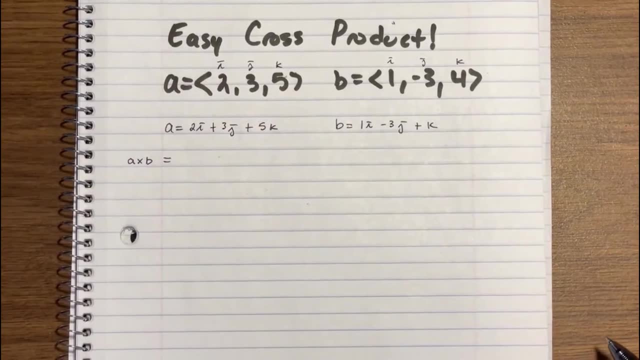 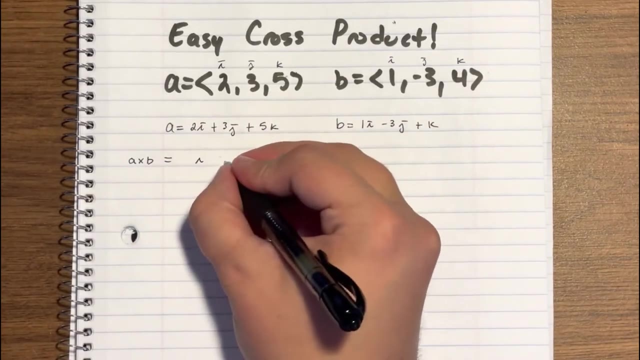 you know imaginary I's, but just forget, those exist right now Anyway. so this cross product, right, What you do is you first you write out I, J and K, So we just have to know we're working with those. So to remind us, 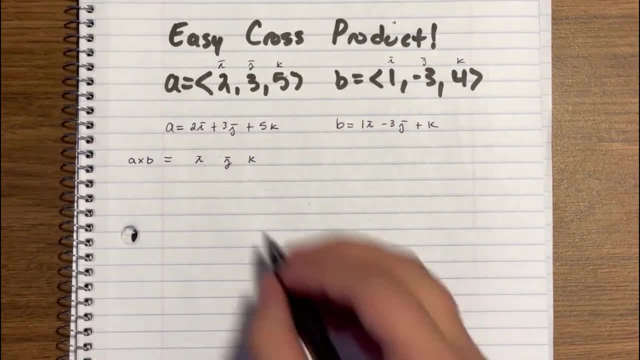 to like make sure the math works. we're going to write out I, J and K. That's going to be our first row of this guy. We're actually going to make like a square, Then under that you do the. 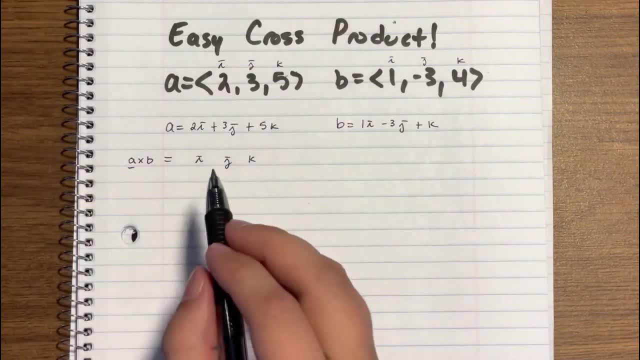 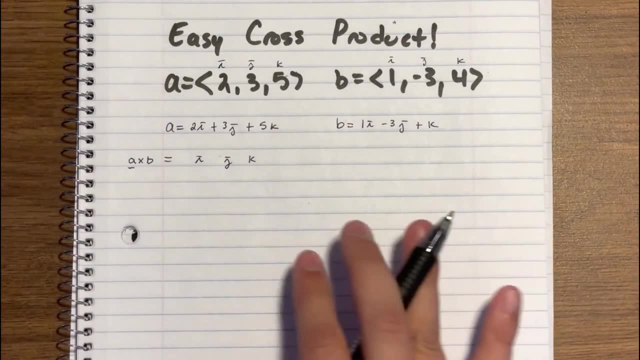 one that's on the left, You always start with the one that's on the left for the cross product. So cross product does not. it's not commutative, So the order of the terms matters. It's not like two times three is the same as three times two. A cross B is not the same as B cross A, That's. 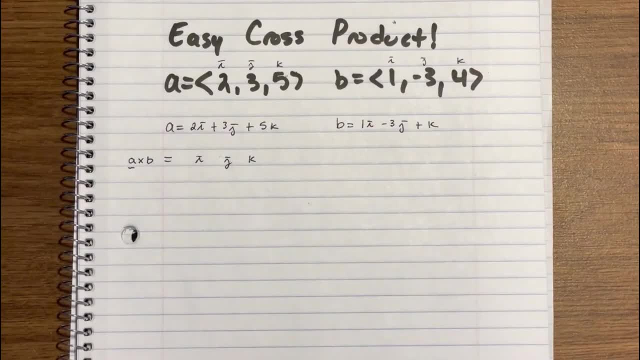 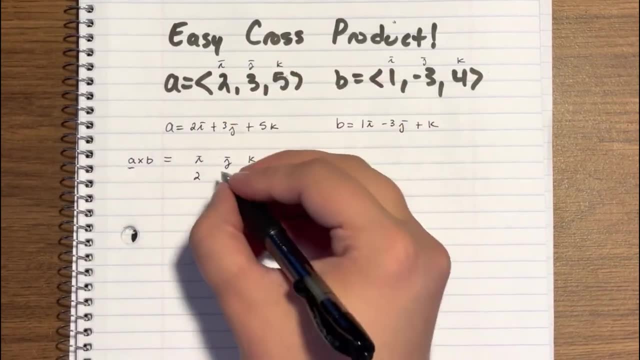 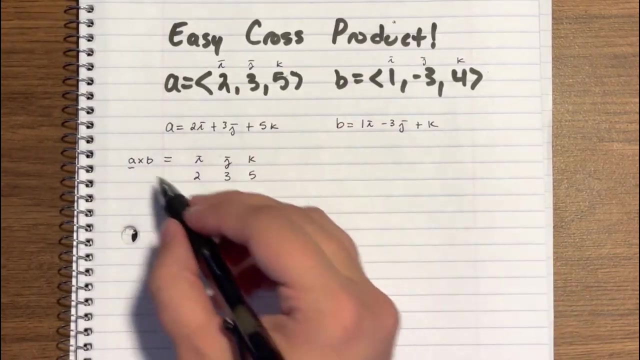 they're actually going to be like opposite. so you would like totally mess up if you did that. So start with the one on the left. We do the I term under I, J term under J, and then the K term under K. There that's A, two, three, five, Then under. 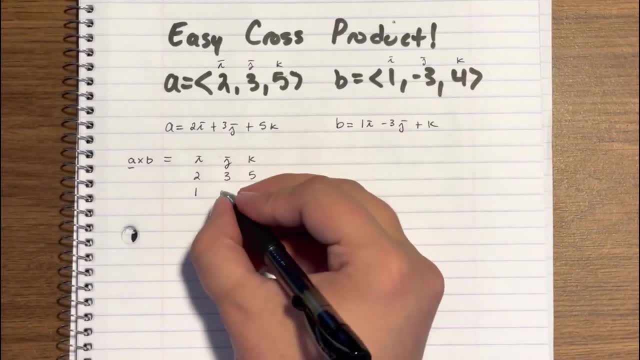 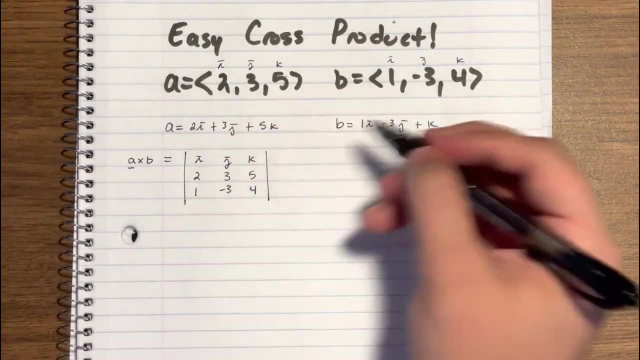 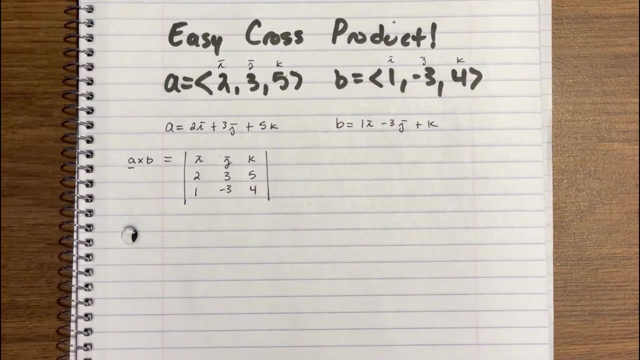 that you put B, I term, J term, K term. Then we just draw these little lines just to make sure we keep them in this box. That's really cool. This actually makes a matrix which I'm not going to explain that right now. but 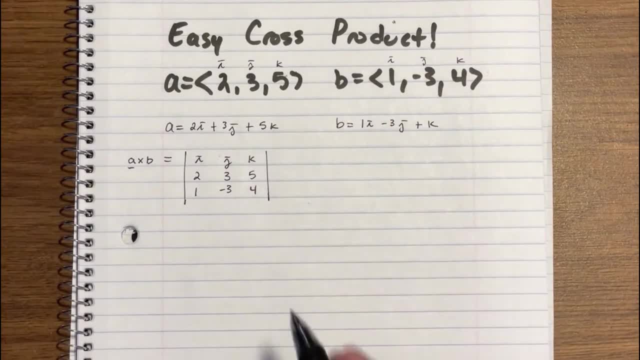 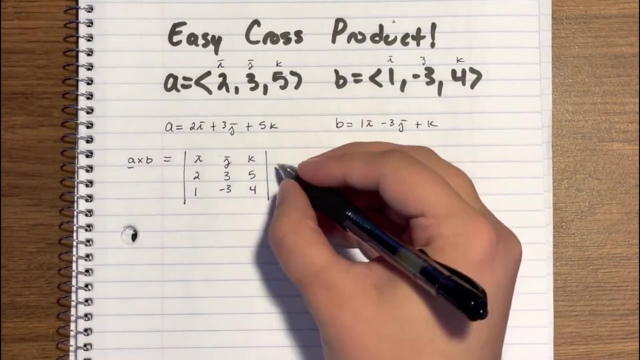 there's a way to solve this using matrices, which we're kind of doing, but this is a shortcut to do that. So after you make our little matrix, we're going to add on a bit to it. This is where it kind of differs from the matrix solution. So after that we're going to add another I and another J. 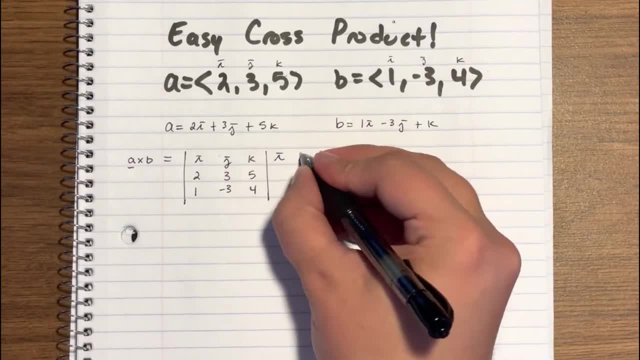 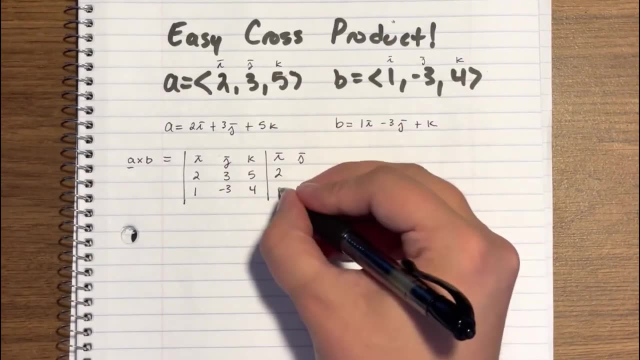 column, And because we're doing the I term, we're going to add another J column And because we're doing the I's again, we take the AI and the BI And then for the J's, we take the AJ. What's up, AJ? 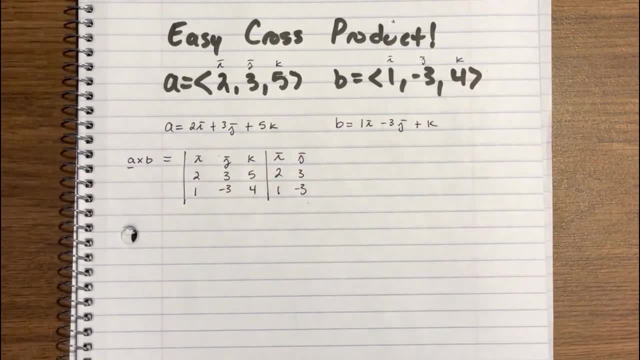 And the B. I'm not going to say that one. Yeah, So yeah, after that we're going to do this. So the next step is to draw diagonal arrows across the square. You can either start at the top or the bottom. I'm going to just start at the bottom. I started at the bottom. Now I'm here, I'm going to. 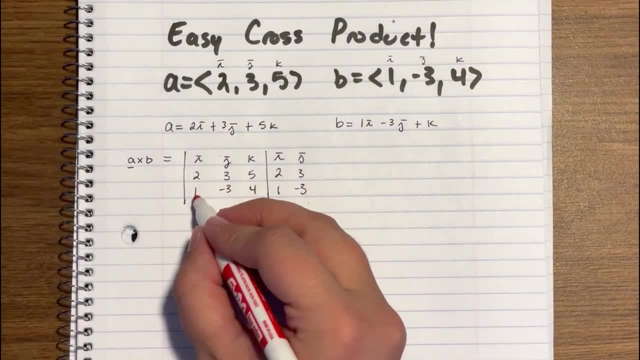 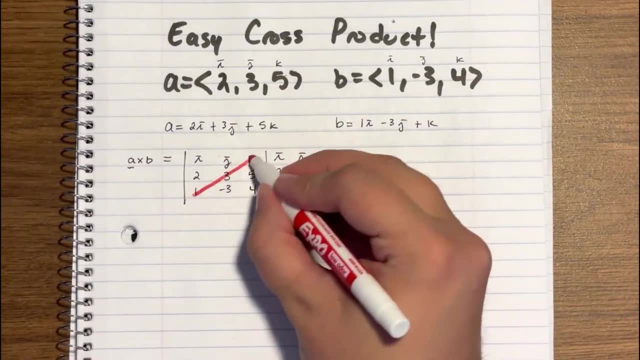 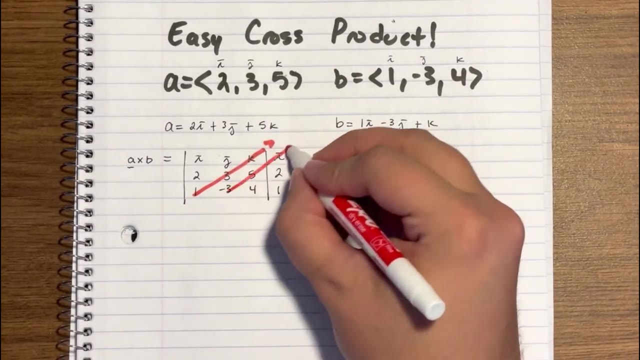 start here And I'm wondering what to do next. So start in this bottom left corner. You see this one, So you can draw a diagonal line from the one up to that K and draw like an arrow through it, Then go to the next term, Negative three. we're going to draw that up through the I. 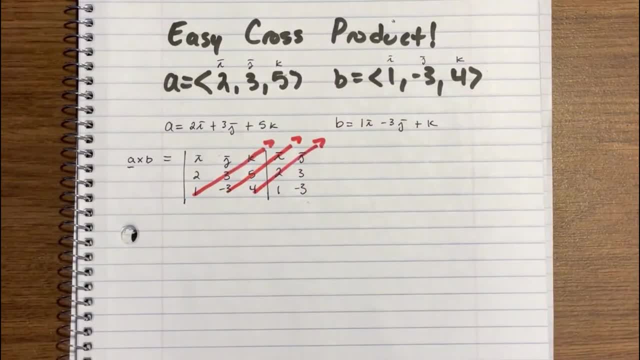 And then that four draw it through the J. All right, cool, And we're going to call these our negatives. So these are our negative arrows. That's also really important. Start at the bottom. So I have like some way to remember this. Start at the bottom. It's negative. 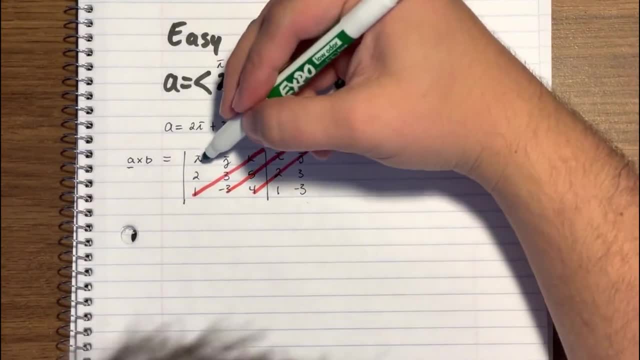 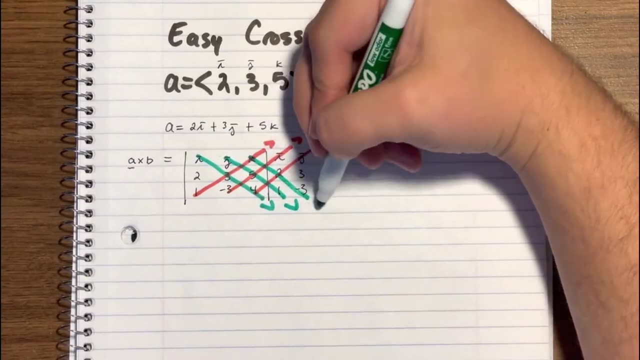 And then if you start at the top, like at this I, you can kind of guess. So it's actually going to be positives. So here we go, Do the same deal, Diagonal from the top. I'm using colors, so it's. 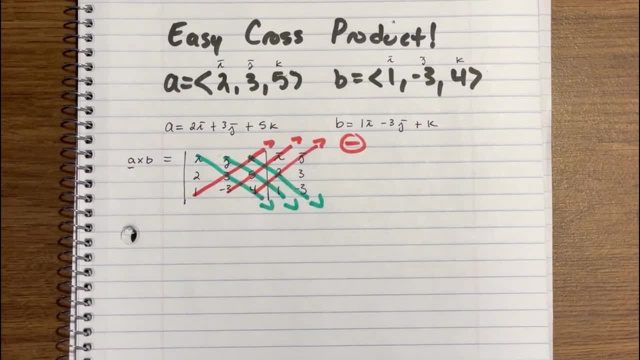 easier to tell. You can just, either, like you can use a pen or something, or like just have some way to draw the lines. Make sure you can still read your numbers Drawing the lines. I've messed up and, like, made it unreadable before. 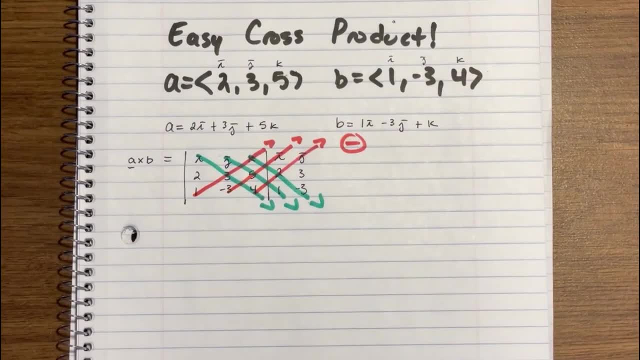 But yeah, just be careful. Oh yeah, And these are our positives, Not a one It's positive. There we go, There we go. See, I got all the moving parts All right. So then you want to. 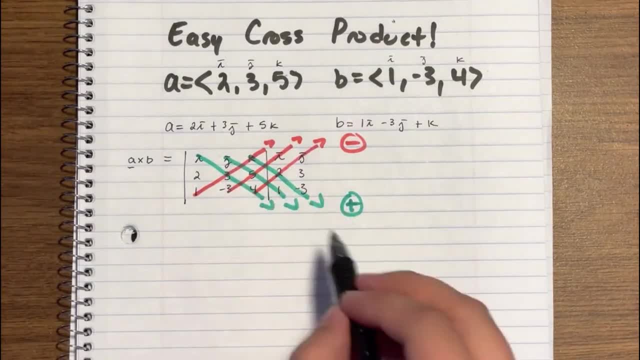 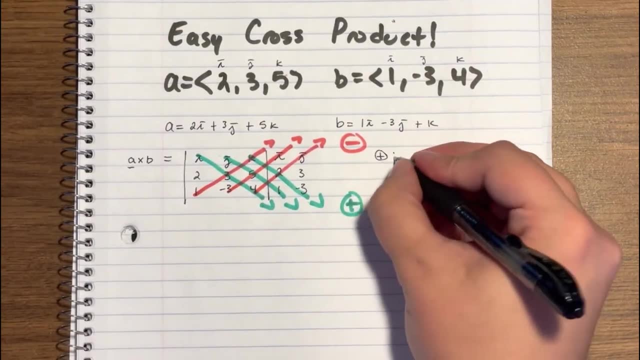 There's a point to doing this. So you actually are going to multiply across these lines and I'll show you how to do that. So let's start with our positives. I like to start with the positives just because they're positive and I'm a positive person, So I'm going to pick those. So let's see. 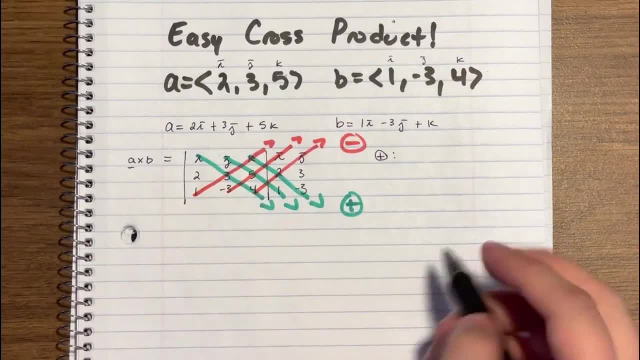 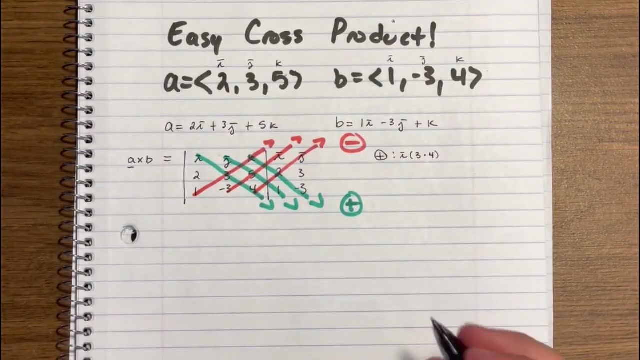 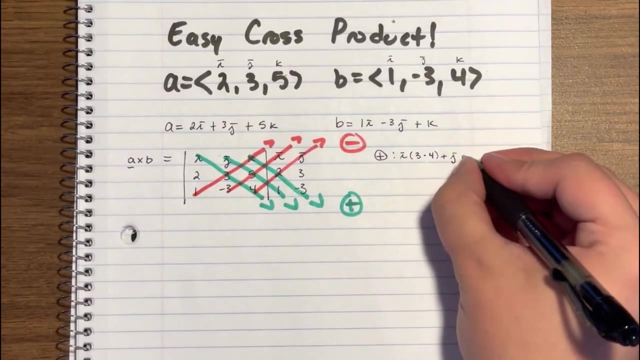 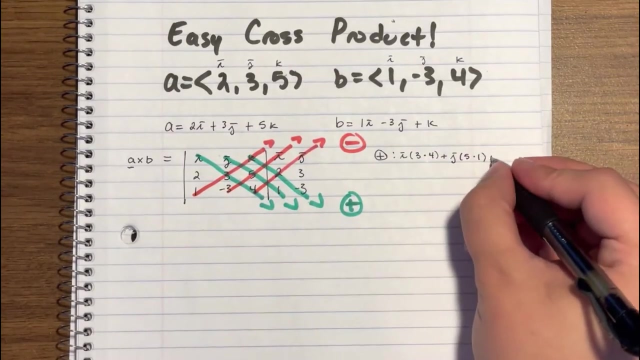 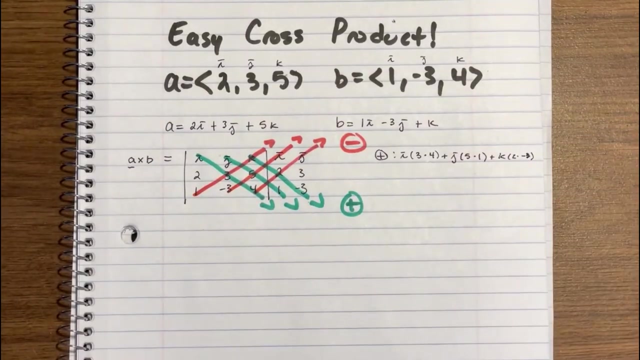 We're going to go I times three times four. Cool, That's simple enough. And then J- You're going to add that to J times five times one. See that. Finally, K times two times negative three. That's a three, I hope you can tell. Then you want to multiply these out. I'm doing this step. 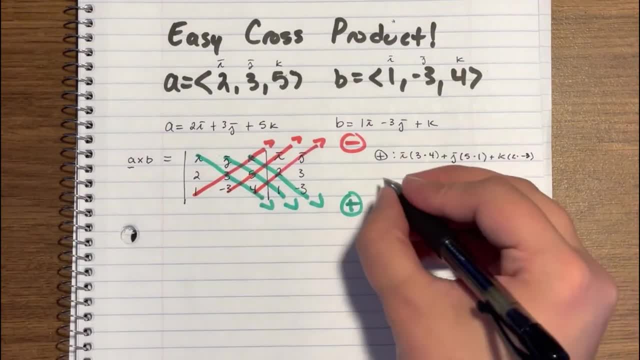 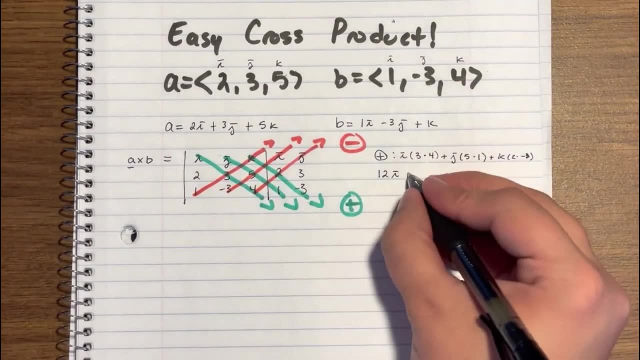 by step, just so you guys don't miss anything. I don't want to feel like you know, don't you guys? to feel like I'm skipping a step, because you can do a lot of this in your head and you can jump to the next step. But for this example, I want to write it out So you guys see: Right, So we got. 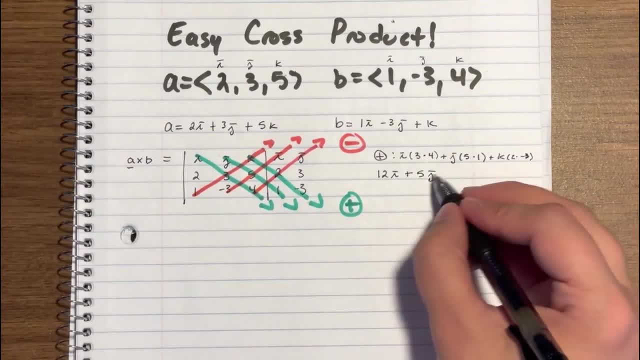 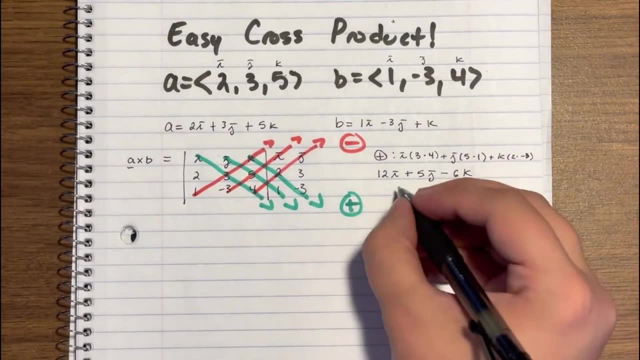 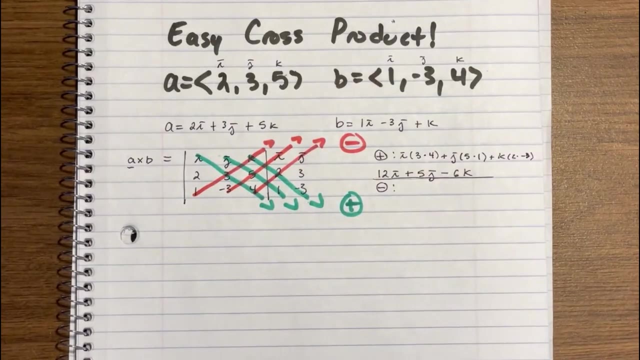 three times four is twelve, Twelve I. Five times one is five J, And then two times negative: three minus six K. Cool, That's our positives. You can like draw a little line under that. Then we got our negatives, So negatives, All right. 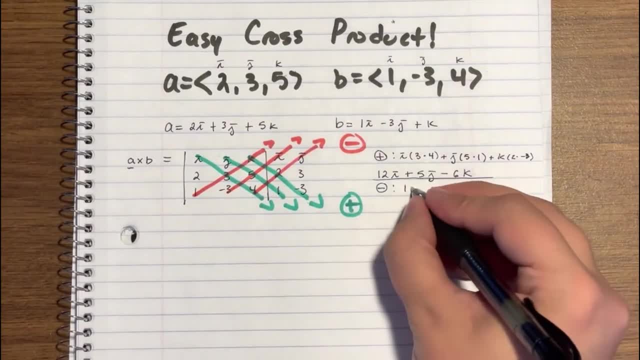 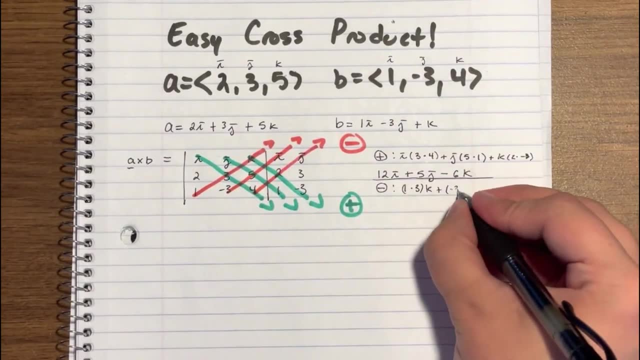 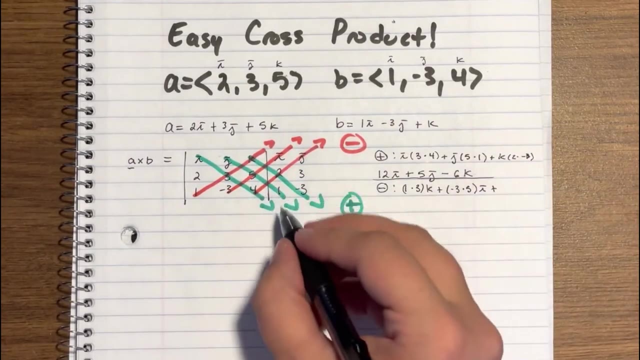 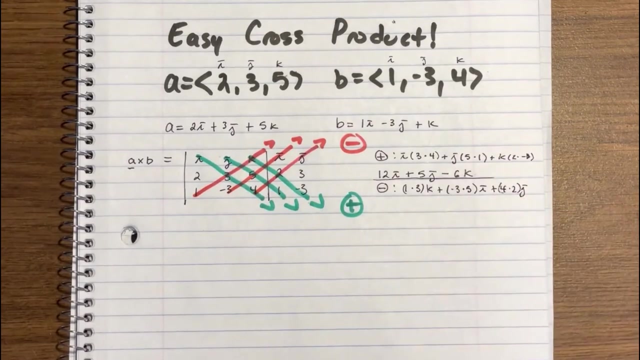 Start at the bottom. Now we're here. One times three times K, Then add negative three times five times I, Then we add four times two times J. All right, Now let's combine those. I like to write it in the order of like: I, J, K. 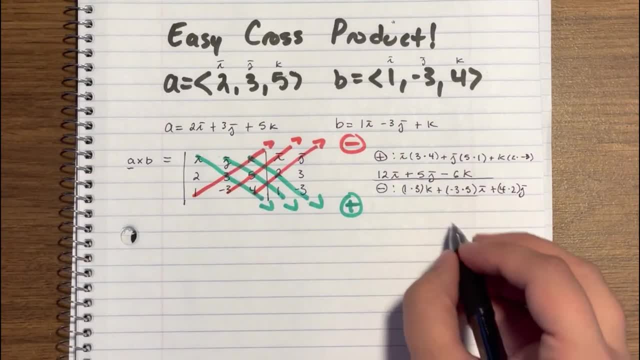 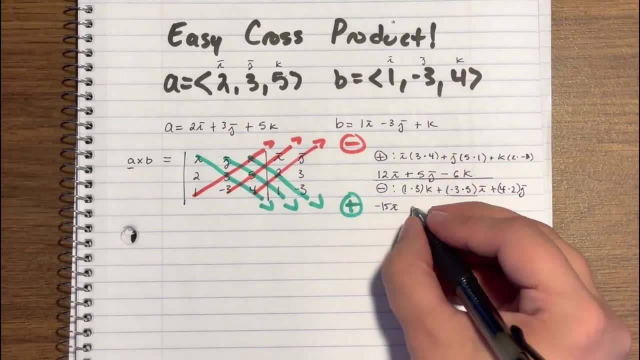 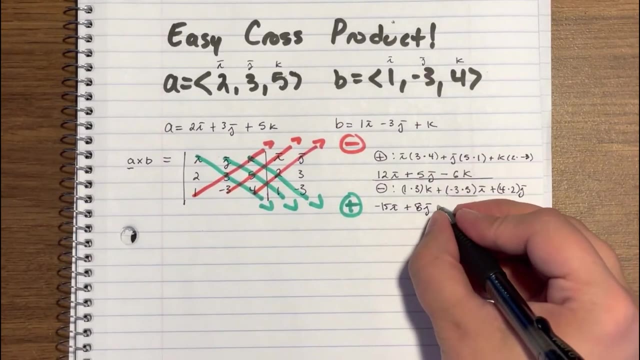 I. just that makes a lot of sense to me. So let's do this first: Negative three times five is minus fifteen I. Then we got four times two times J is eight, J, That's eight. Then we got one times three times K Plus three K, Cool. 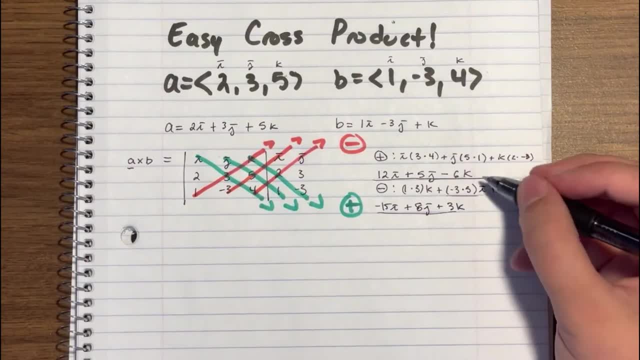 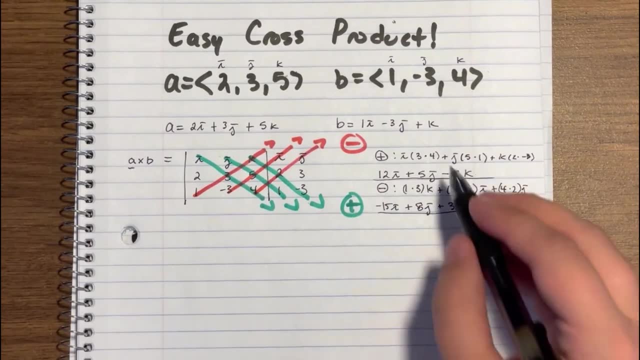 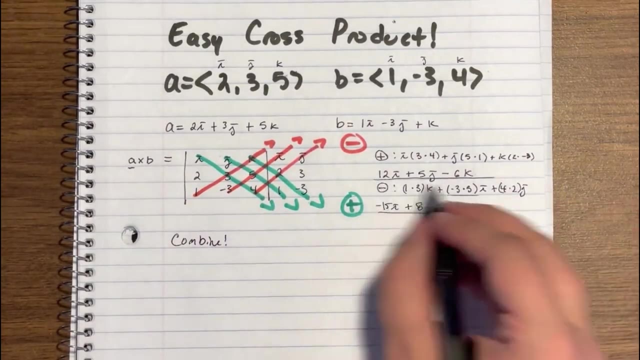 Now we have these two Like halves. These are like halves of our solution. We got the positive and the negative half. OK, so then we got our positive and our negative. Then we take them over here and combine them. So we've got our positive up here. 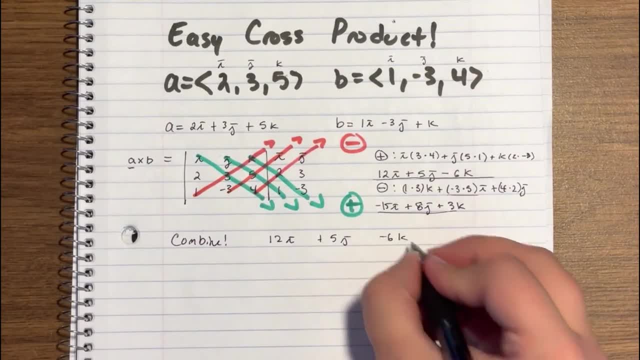 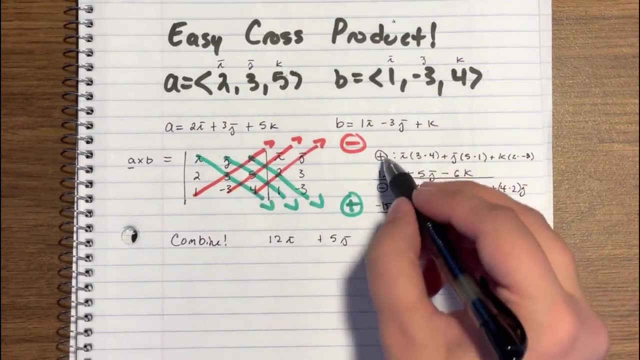 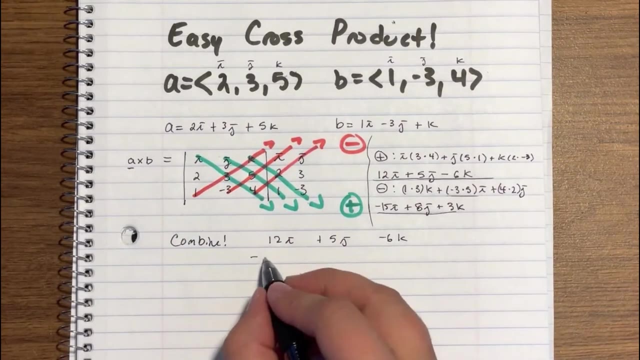 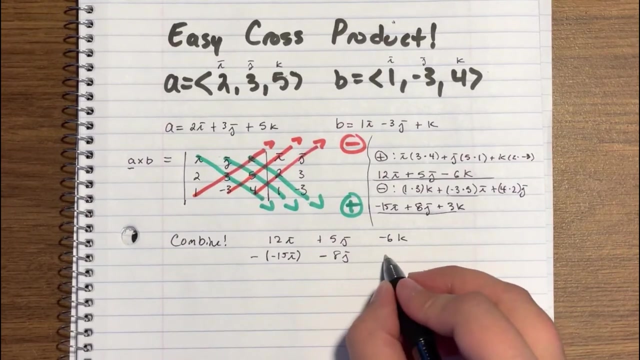 And then we subtract our negative. I know this is confusing, but just look at the signs over here. So we got our positive, Then subtract our negative, So we minus Right. So we got minus this term, minus this term, minus this term.